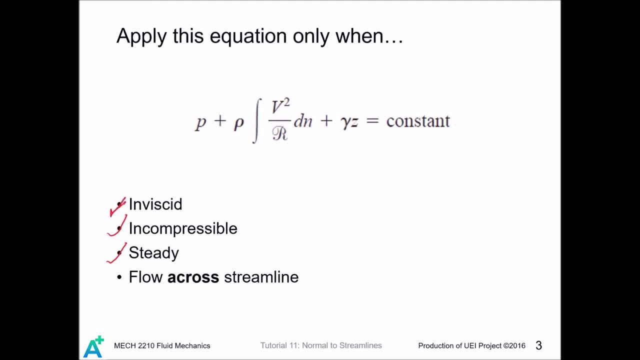 steady and viscous effect can be neglected, And this equation is for a cross streamlines, not a long streamlines. If a long streamlines is available, then we must apply the Bologna equation. Now we do a quick example to illustrate how to use this equation. 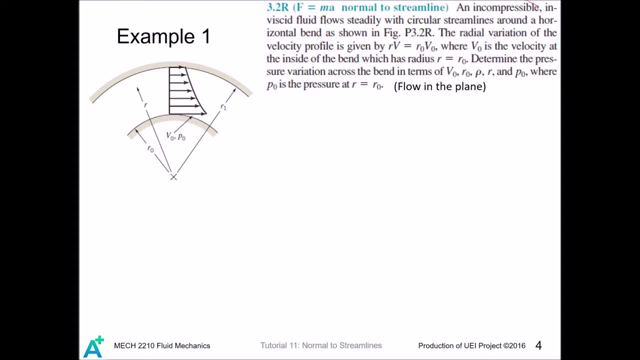 So we first make sure that we can apply this equation. The flow is incompressible, infiscus, steady, and we have to determine pressure variation across streamlines. So we can apply the formula We write down: C plus rho, integrate 3 squared divided by R, dA plus gamma z equals C. 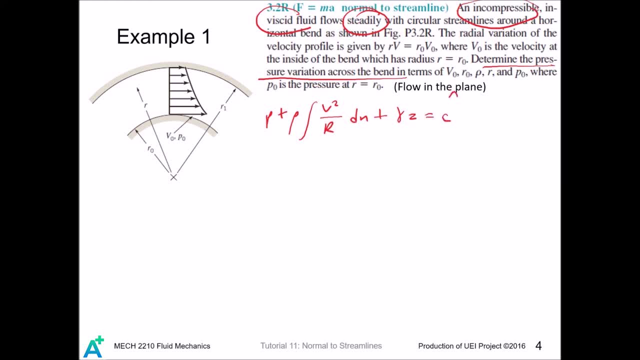 In fact this flow is flow in the x-y plane, So there is no gravity here and we can neglect this term And look at here: We are provided that R times 3R equals R naught 3 naught, So we have 3 as a function of R equals R naught 3 divided by R. 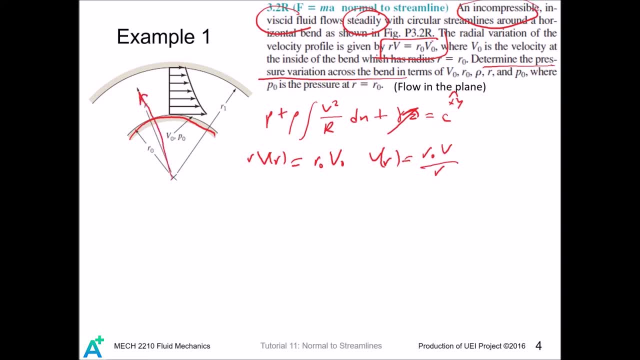 We also observe that R points radially outward And for any loss we can apply this equation. We have N points radially inward, So we have minus dN equals dr. So looking at this formula and if we take reference about this arc, 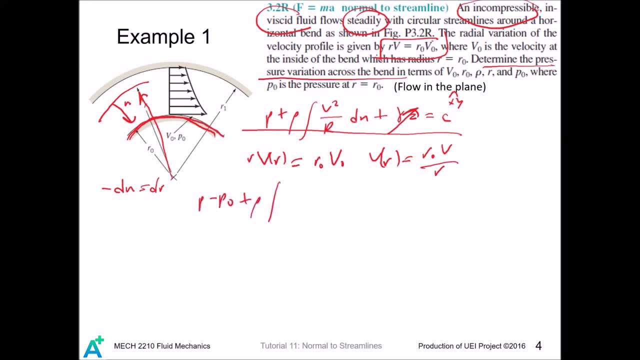 we have P minus P naught plus rho R, integrate from R R naught. R is just R minus dr equals 0. And we substitute in the expression for V And we simplify a bit, And this thing equals 0. So we have P as a function of R or 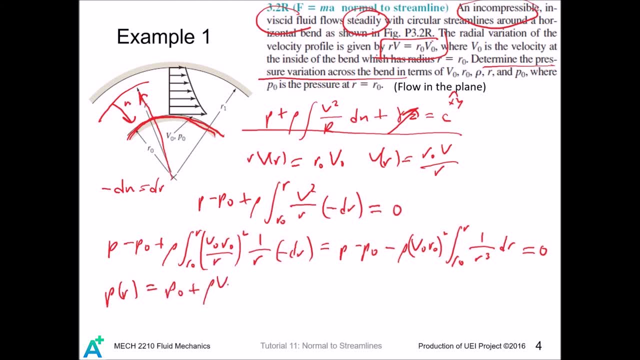 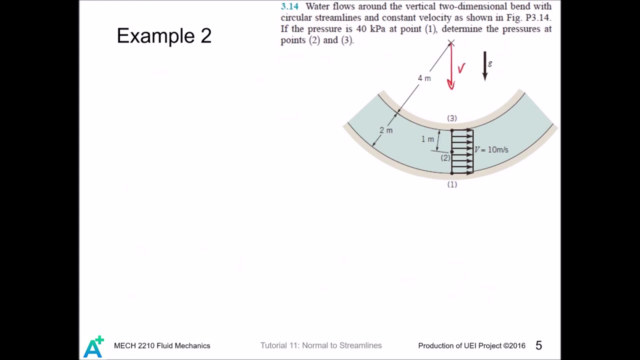 equals P naught plus rho V naught, R naught squared divided by negative 2.. And this thing equals P naught plus rho V naught. Yeah, and we do. the next example: let's set the r-direction like this. and again, if we